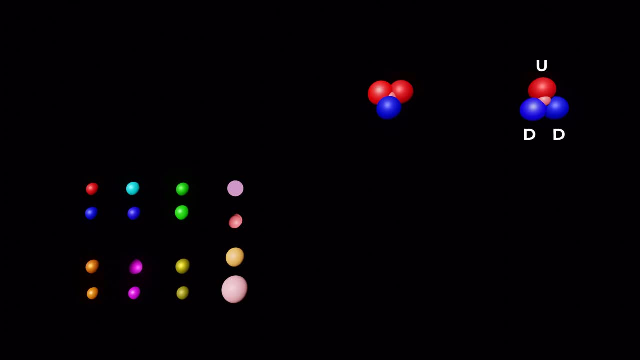 while a neutron consists of two down quarks and one up quark. Particles with masses equal to or greater than that of protons are called baryons, and both protons and neutrons are baryons. They are composite particles made up of quarks. 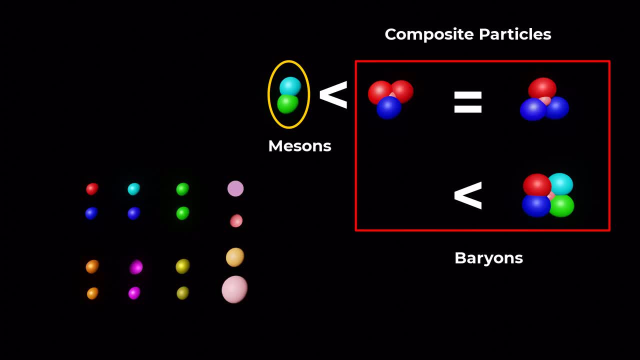 Particles with masses less than that of protons are called mesons, which are made up of two quarks, a quark and anti-quark pair. Mesons and baryons are collectively known as hadrons. The matter outside the nucleus of an atom is made up of leptons. 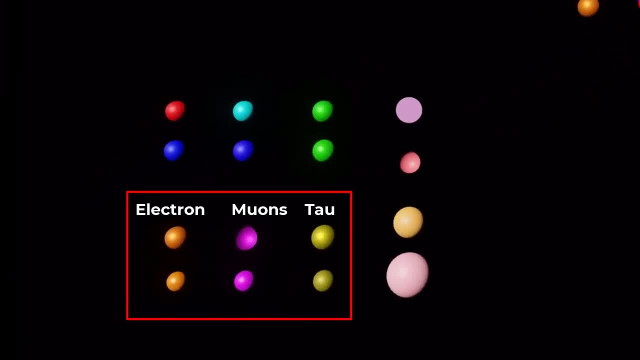 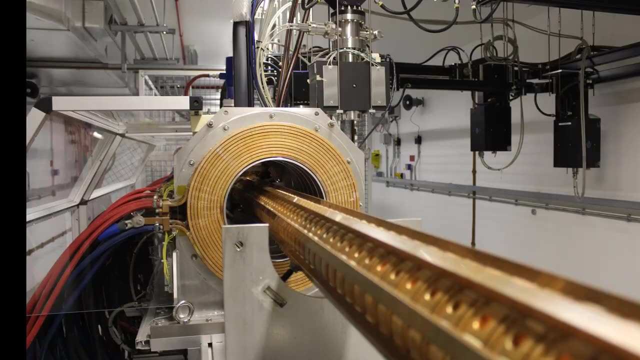 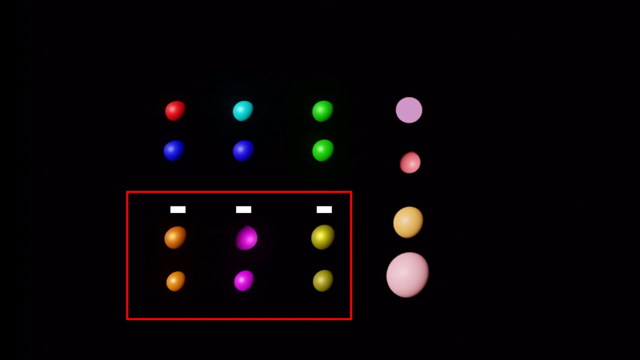 The most well-known leptons are electrons, muons and taus. Muons and tau particles are typically produced in high-energy processes, particles, accelerators and certain radioactive decays. Each of these types has a negative charge and a distinct mass. 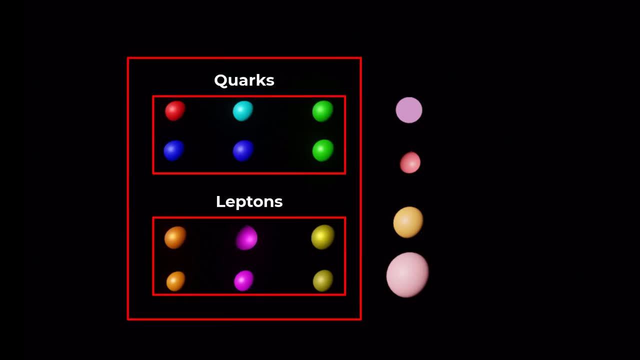 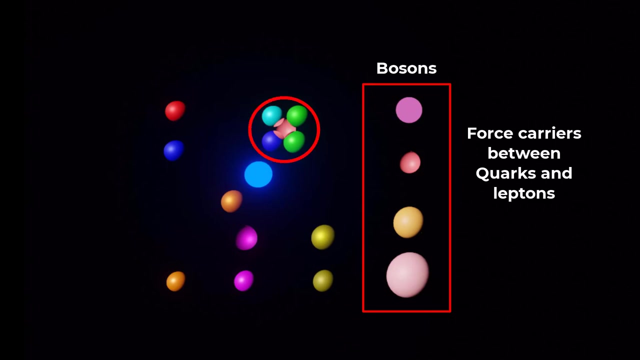 Leptons and quarks are collectively called fermions, which are indistinguishable spin-half particles that obey the Pauli exclusion principle. Bosons are particles that act as force carriers, causing interactions between other particles like quarks and leptons. 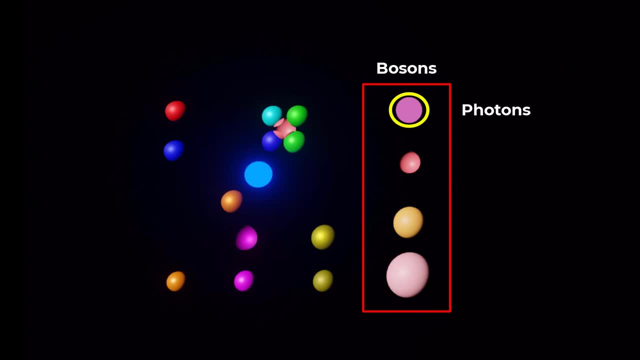 The most well-known bosons are photons and gluons. Photons cause electromagnetic interactions, while gluons act as the force carrier between quarks, creating one of the fundamental forces of nature: the strong force. All the bosons have either zero or integer spin and don't obey Pauli exclusion principle. 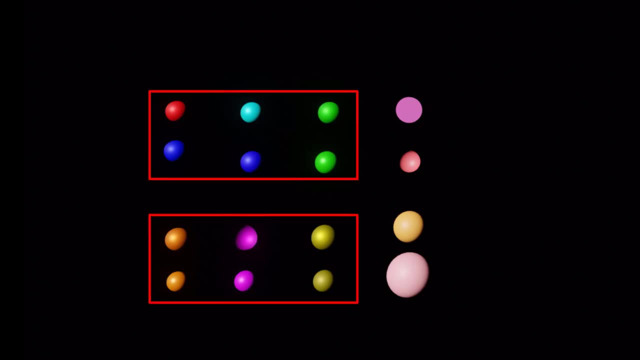 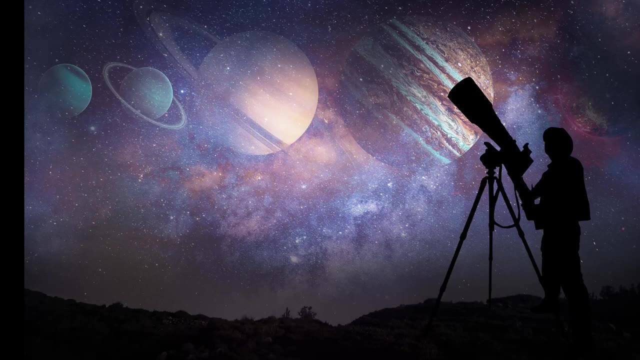 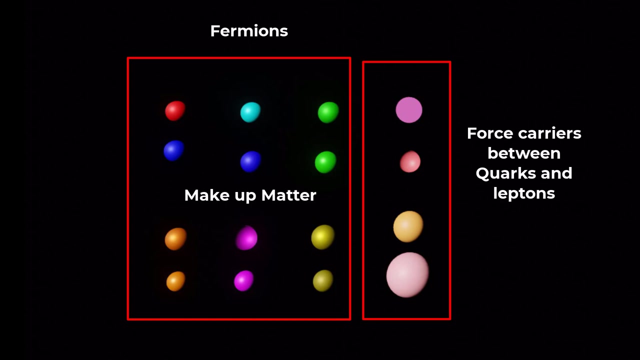 In conclusion, from quarks and leptons to bosons and hadrons, these tiny particles come together to form everything we see around us. The particles that make up matter are known as fermions, and the particles that carry forces between other particles are known as bosons. 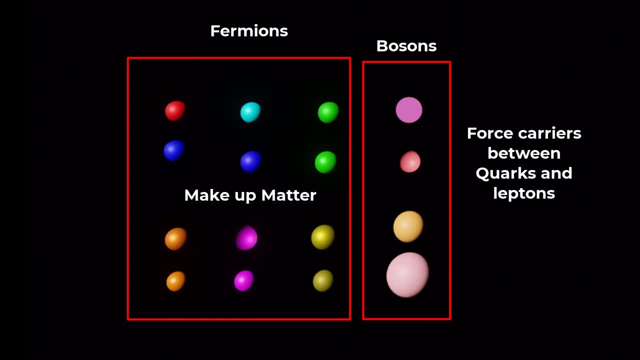 We hope you've learned something new about the building blocks of our universe. Thank you for watching.